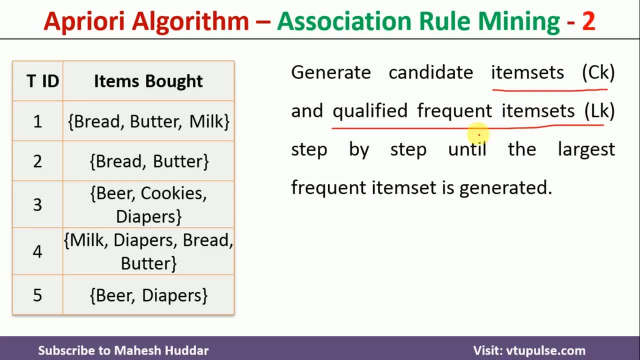 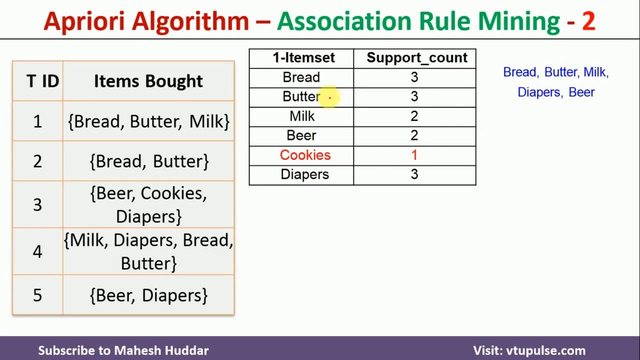 is having minimum support. So I will explain how to do it step by step. In this case we have five unique products here, that is, bread, butter, milk, diaper and beers. So we will write those particular thing in the first column of this table as one item set. 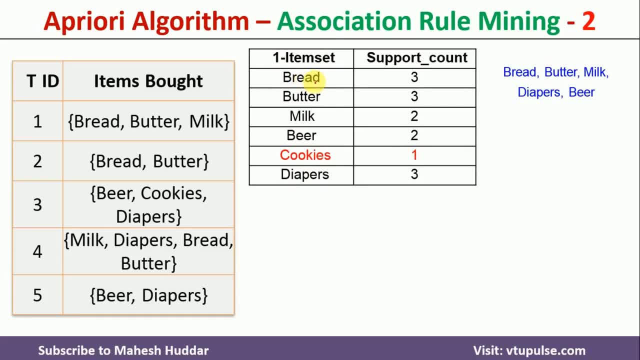 Then we count the number of times a particular product was bought. For example, bread Bread was bought once, twice, thrice here, So that is three in this case. Similarly, butter Butter was bought first time, second time and then somewhere here it's a third time, So it is three here. Similarly, 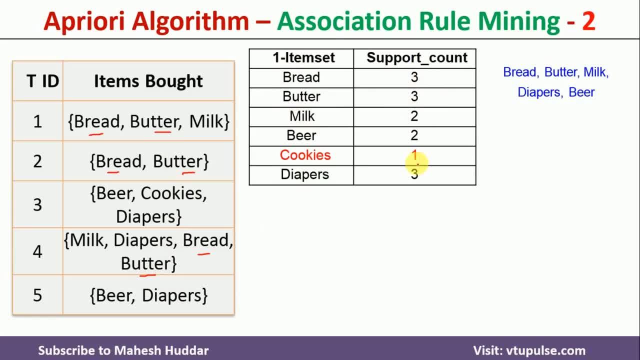 two times a particular item was bought. And then we need to write in the second column that is the support count. So this is one item set table. From here we need to generate the one of frequent item sets. For that reason. first we need to do some simple calculation. 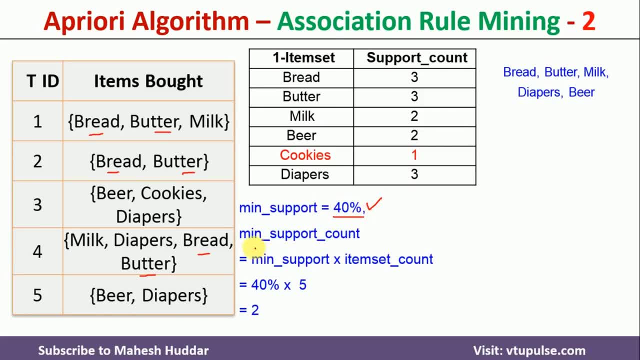 The minimum support given to us is 40%. So the minimum support count is equal to minimum support. that is, 40% multiplied by item set count. That's how many items are there? There are five items. answer is 200 percent. that is nothing but 2. 2 should be the minimum support count, then only. 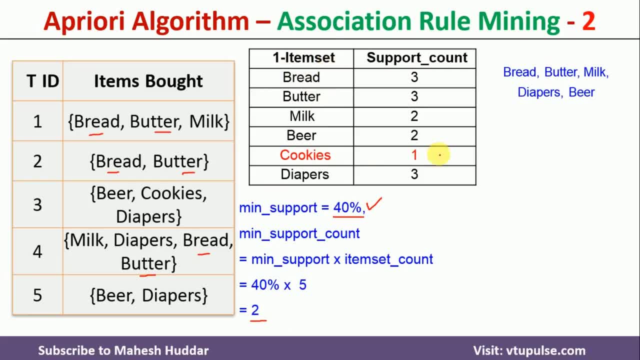 you can say that one item set is a one frequent item set. so in this case, except this, cookies, all are one frequent item sets, those i have written in this particular table. that is nothing but one frequent item set. now, if we look at this particular one frequent item set, we have five. 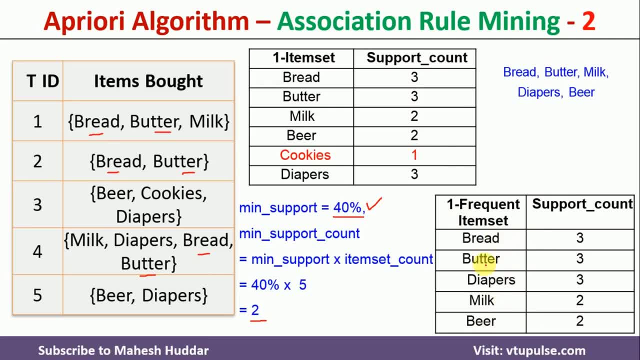 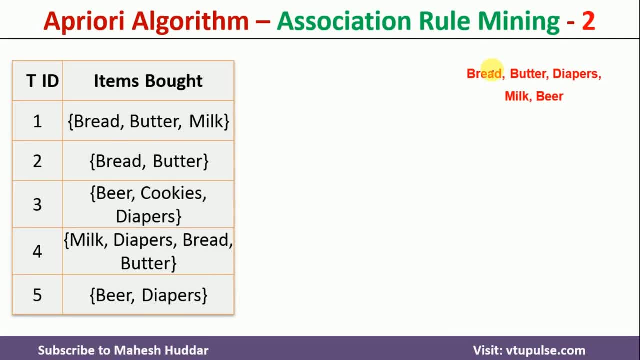 unique items again, we need to generate two item sets here. so these are the five items we have. so two item sets are like bread, butter, bread, diaper, bread, milk, bread, beer. that's a five first, five combinations. next one is butter, diaper, butter, milk, butter, beer. the next are diaper, milk, diaper. 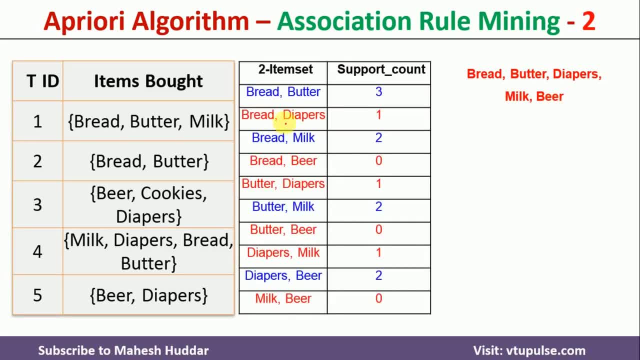 beer and the last one is milk beer. so those are the combinations i have written here. you, once you write this particular combinations we need to find, or can say that we need to count, how many number of times these two items were bought together. bread and butter, if you see here. 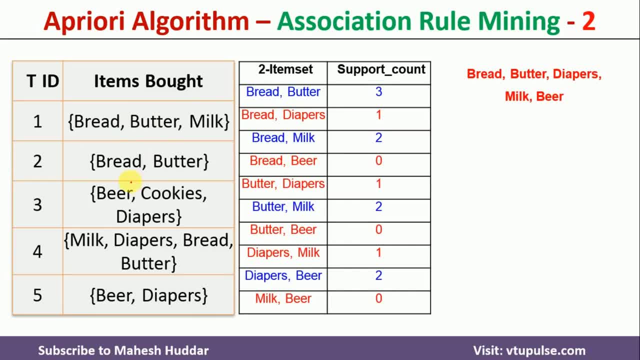 it is bought first time in this first transaction, second time it was bought and then in the fourth transaction. also these two items were bought together. so the answer is three in this case, similarly, bread diaper. bread diaper was not bought here. i think in the fourth transaction bread is present and diapers is present. 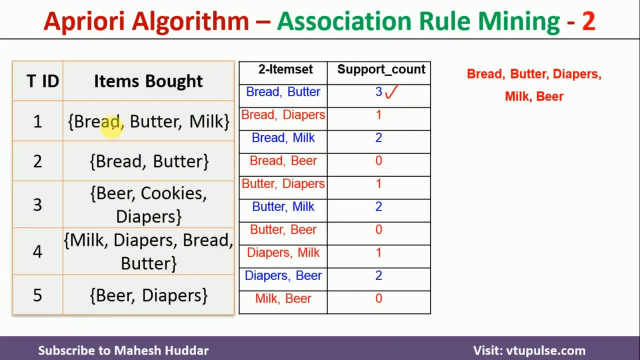 so it is bought only one time: bread and milk. bread and milk is present in the first one. bread and milk is present in the fourth transaction, so it is two. similarly, we have to find the support count for each and every item. that is nothing, but how many number of times these two items were bought. 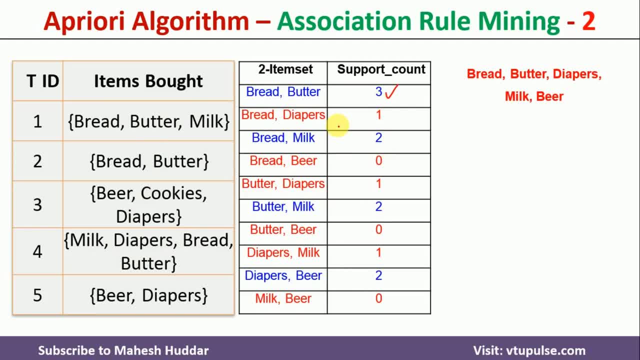 together and then we need to select the two item sets which are having minimum support count of two or more. so in this case we have only four possibilities, that is, bread, milk, bread butter, buttermilk and diaper beer in this case. so these are the four possibilities now from this particular two frequent item sets. 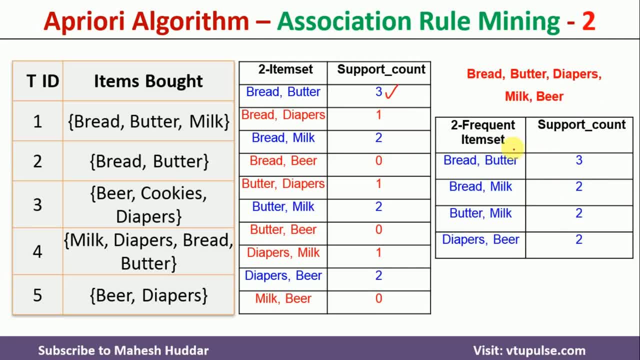 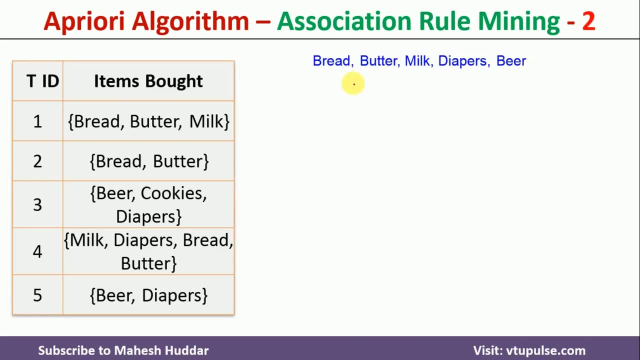 we need to generate three frequent item sets. for that reason first we need to write three item sets. so first we identify what are the unique items are present here: bread, butter, milk, diaper and beer. all five are unique items here. from this particular five unique items we need to generate 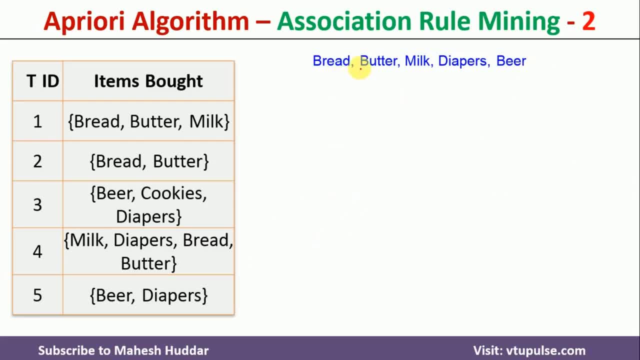 three item sets in this case. i will show you one example. how can you do this? one is bread. we can start with bread here: bread butter, milk, bread butter, diaper, bread, butter, beer. so bread and butter is poor. so bread, milk, diaper, bread, milk, beer, bread and milk is over bread, diaper, beer. so bread, butter, bread, milk, bread, diaper. 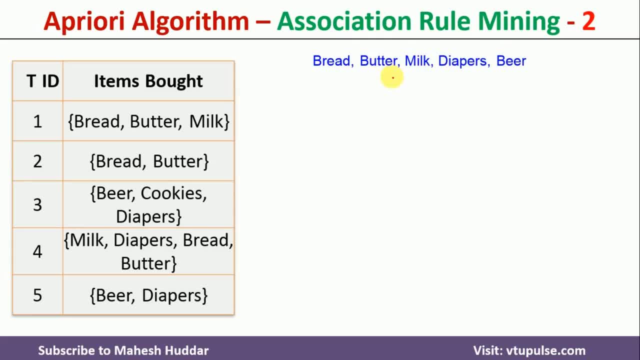 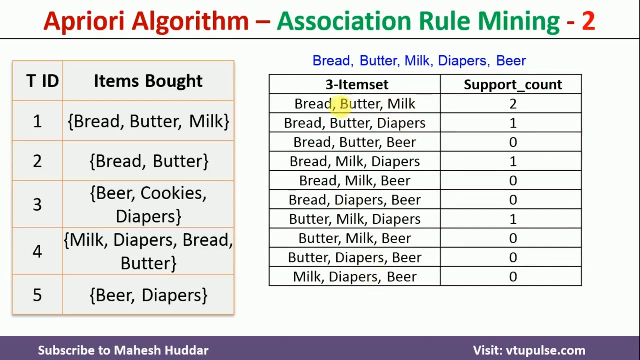 are over. now I will come with this one: butter milk diaper, butter milk beer and then butter diaper beer. that's a ninth possibility, and the tenth possibility is a milk diaper beer here. so totally, we have 10 possibilities for this particular 10 possibilities, we have to again. 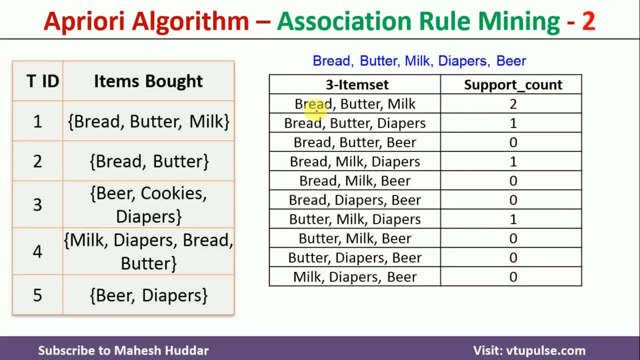 count the minimum support, for example, how many number of times these items were bought. that is nothing, but the support count. bread milk butter. bread milk butter is present here. this is the first time bread milk butter is present one more time here, so it is two, similarly, if you go with. 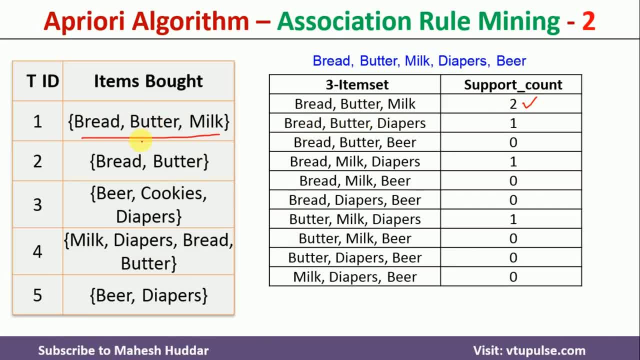 the second one, bread butter diaper. bread butter diaper is present in the fourth transaction. you can see here bread butter diaper is present. anywhere else it is not present, so it is only one. so similarly we have to do it for all combinations and then write that particular support count in. 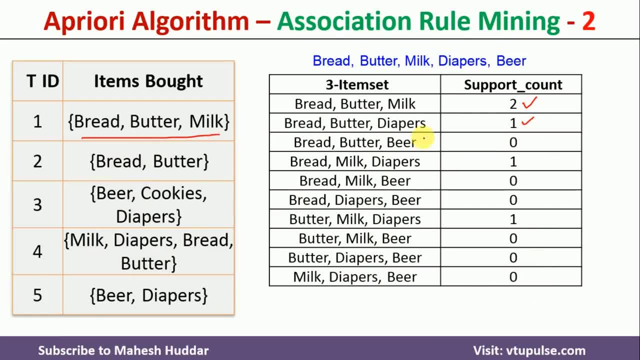 the second column. next we have to select the three frequent item set which satisfies the minimum support of two. in this case, we have only one, that is a bread butter milk with a support count of two in this case. now coming back to the next one, that is, once you find the free three frequent item set, 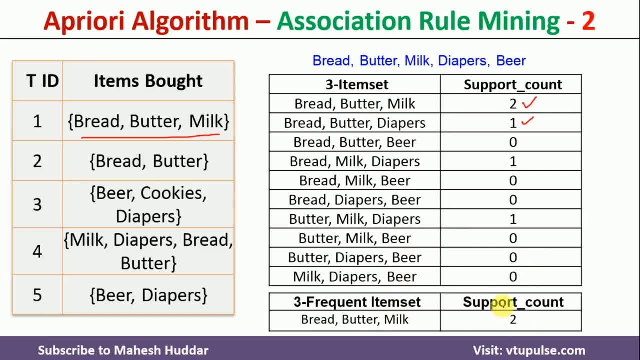 we need to check whether it is possible to write four frequent item sets in this three frequent item set. we have only three items, so definitely it is not possible to write four frequent item sets, so we have to stop here and that is generating the frequent item sets. now we need to write the. 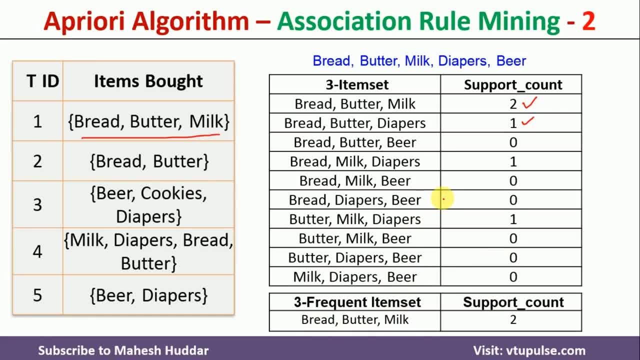 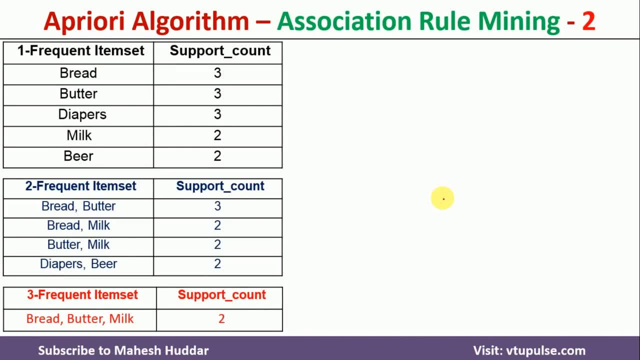 association rules and select only those association rules which are strong based on the confidence percentage. now, if you want to generate the- what we can say, that the strong association rules, we have to follow this particular procedure. first, we need to note what is the minimum confidence given. the minimum confidence in this case is 70 percent. so if you want to calculate the, 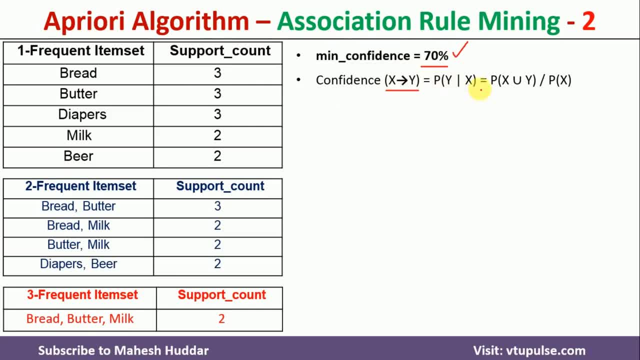 confidence of a particular rule. let us say that x tends to y. it is nothing but the number of times both the products were bought together, divided by the number of times the first item was bought together. but so in this case, uh, how many number of times x and y bought together, divided by the 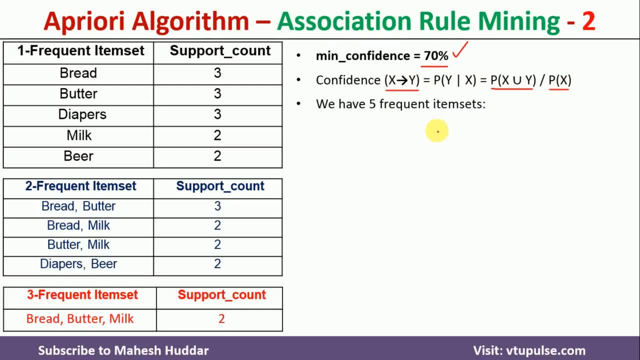 number of time. x was bought here. so first i will write down the frequent item sets. in this case we have four. two frequent item sets are there and one three frequent item set is present. so i have listed all those particular things over here. next i will start with one frequent item set and then i 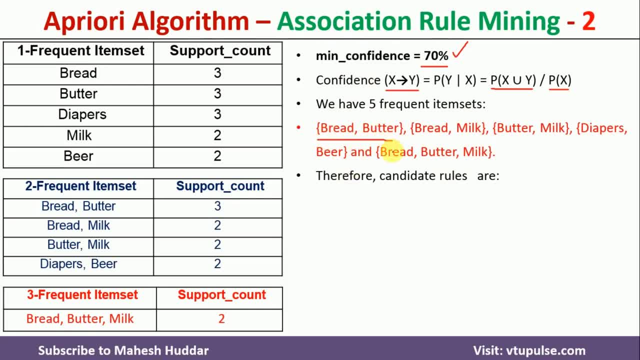 will generate association rule. so first one is this: that is a bread and butter, so bread and butter. the rules can be bread butter or butter bread. these are the two possibilities. now i will check how many number of times bread and butter was bought together, bread and butter was put together. 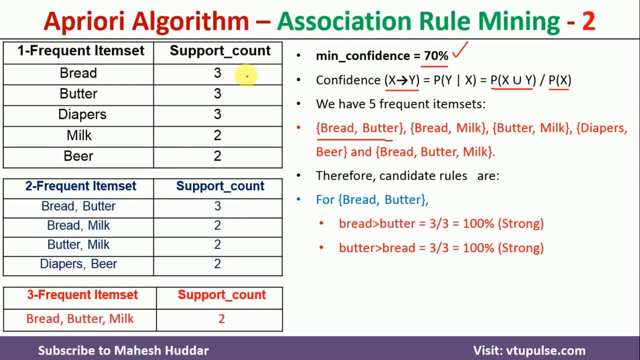 three times, and then i will write down the number of times the bread and butter was bought together. how many number of times bread appears. bread appears three times, so three by three is equal to hundred percent. it is a strong rule in this case. the other side is what? butter, bread, butter. 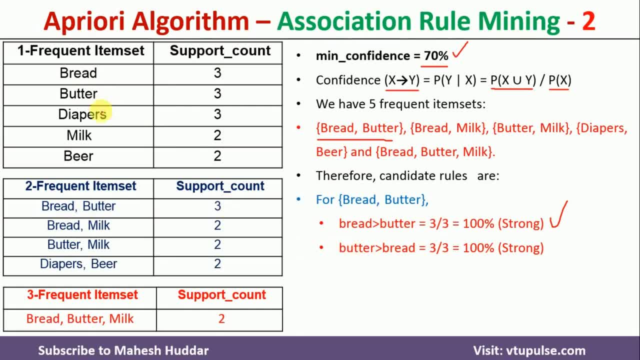 bread is bought three times, and how many number of times butter appears. butter was, uh, appearing three times. it means it was bought three times. so three by three is equal to 100. again, it is a strong rule here. coming back to the next one, that is, bread, milk. bread milk is the one possibility. 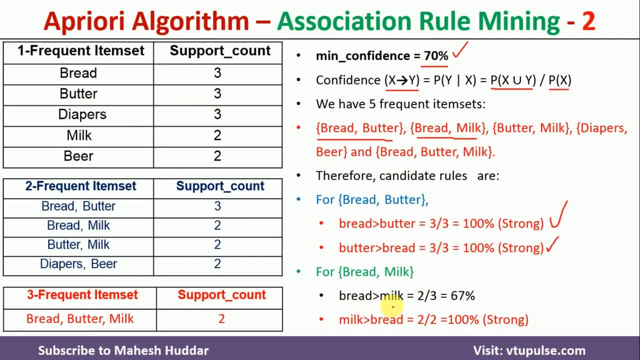 milk. bread is another possibility. bread milk: how many number of times it was bought together? bread milk is bought together two times. how many number of times bread appears is it is three times, so two by three, sixty seven percent. it is not a strong rule in this case. 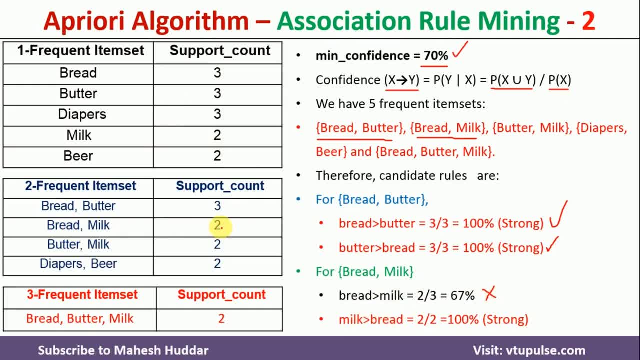 other side is milk bread. milk bread is again bought two times. milk appears two times. two by two is equal to 100 percent. it is a strong rule. coming back to the next one, that is uh, butter milk here, so butter milk or milk, butter, butter milk is bought together. 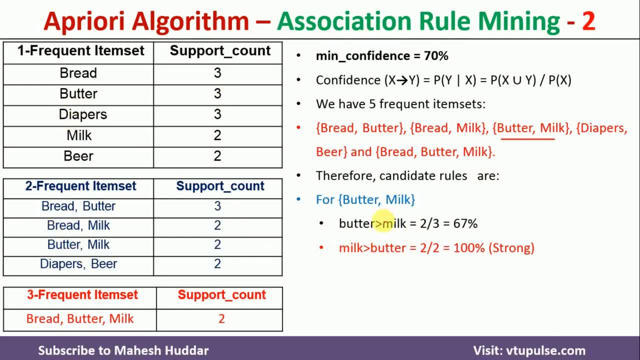 two times. butter appears three times two by three. sixty seven percent. it is not a strong rule. milk butter is the other possibility. milk butter is bought together two times. milk appears two times, so two by two. it is a strong rule in this case. coming back to the next one, that is, diaper beer, this is the next one. 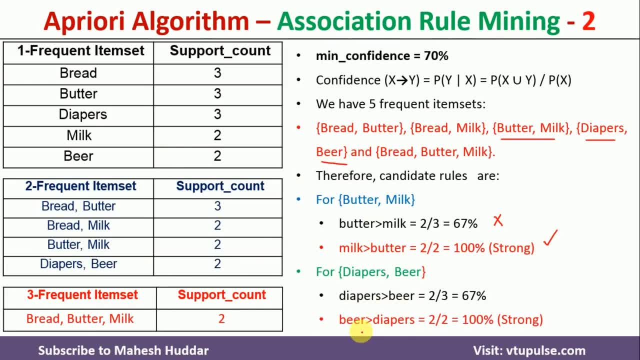 so the first rule is diapers beer. second rule is beer diapers. diapers, beer is bought together two times. diapers appears three times sixty seven percent. it is not a strong rule. beer, diapers, beer, diaper is brought together two times. beer appears two times two by two. it's a hundred percent. it's a strong rule. 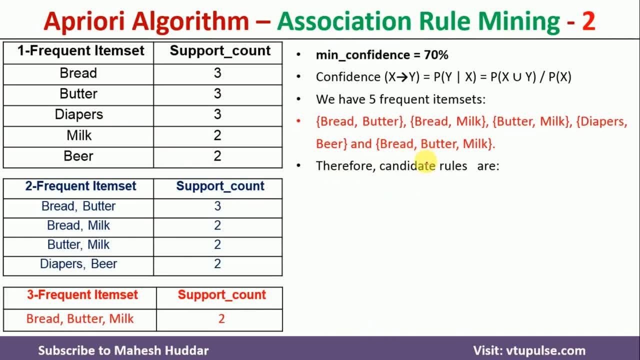 in this case. coming back to the last one, we have left with only one frequent item set, that is, bread, butter, milk. here we have to use simple logic to generate the different association rules. so what we do here is we will write 2 at a time on the left hand side or 1 at a time on the left. 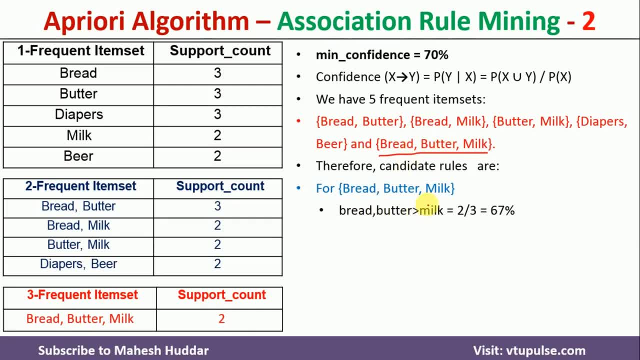 hand side, anyone is perfectly fine. so bread butter. remaining is milk here. so how many times all 3 were brought together? all the time it is 2, only bread and butter 3 times. so 2 by 3, 67%, not a strong rule. so other side of this one is what milk, bread butter or any? 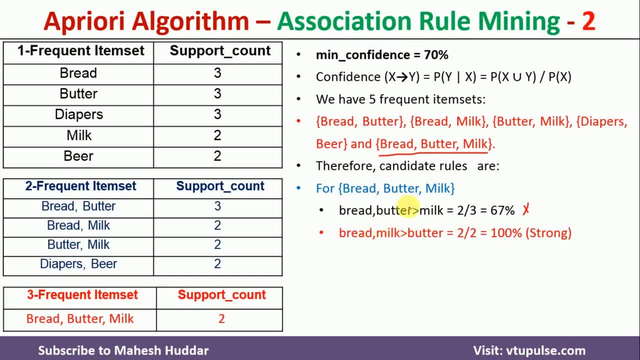 order you can write, but in this case I have written this butter this side, so it will become bread, milk butter. this is one more possibility. all 3 were brought together 2 times and bread and milk were brought together 2 times, so that is nothing but 2 by 200%. and the next: 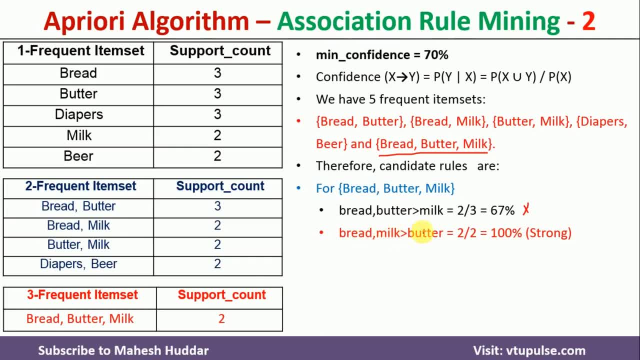 time what we can do is we can bring this particular butter, this side, bread, this side. that's one more possibility. so milk butter bread is the one more possibility. 2 times all 3 were brought. milk and bread butter were bought together, milk and butter two times. so it is be a two by two again here. strong. 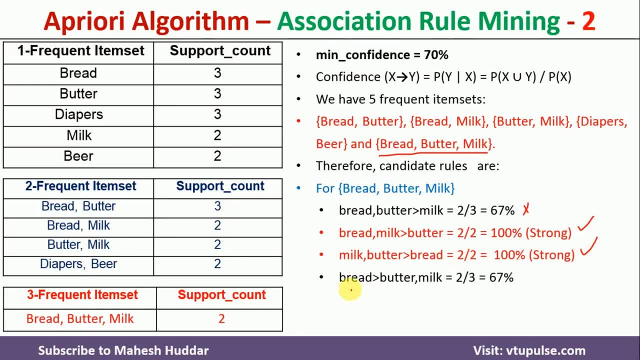 rule, strong rule now. the next one is: what bread, butter, milk. so the opposite of this one. so two by three. uh, it's not a strong rule. next one is: i can bring this particular uh, butter this side, bread this side, and the last time i will bring milk this side and then the butter this side. so 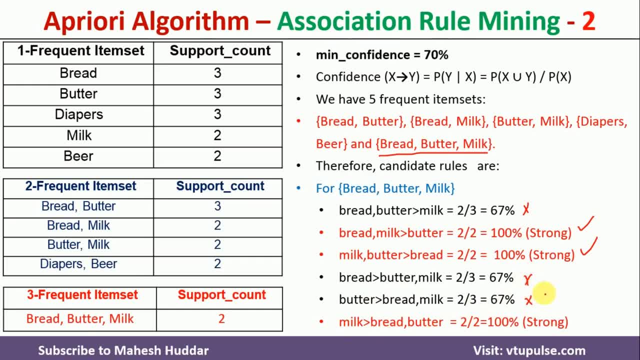 that is the one more thing. these two are, uh, not a strong rules, but the last one is a strong rule in this case. so this is how actually you can generate the association rules and then you can check whether association rule is a strong or not by considering this particular confidence value. 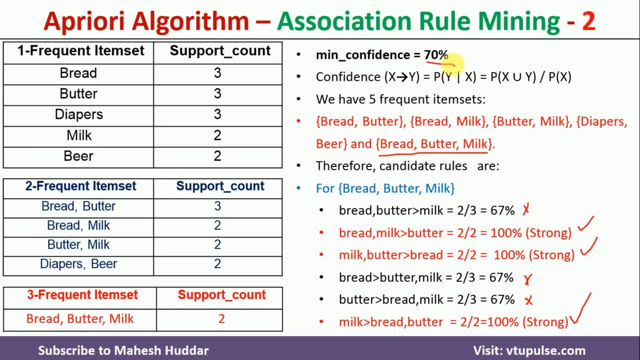 so this is a very simple process with which you will be able to generate the frequent item sets and then you can generate the association rules and then select the association rule based on the minimum confidence in this case. i hope the concept is clear. if you like the video, do like and share with your friends. press the subscribe. 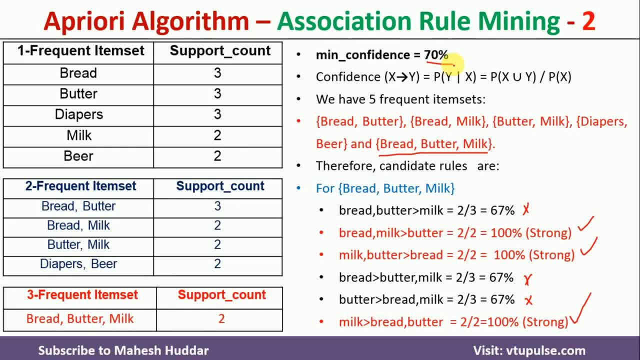 button for more videos. press the bell icon for regular updates. thank you for watching.